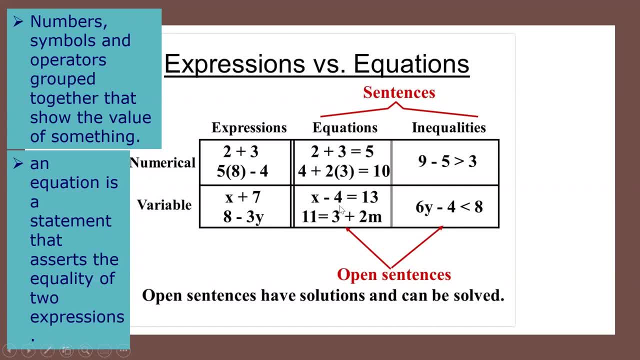 So 2 plus 3 and 5 are equal, x minus 4. And 13 are equal for a specific value of x. Now, in inequalities, an inequality is a relation which makes a non-equal comparison between two numbers or other mathematical expressions. 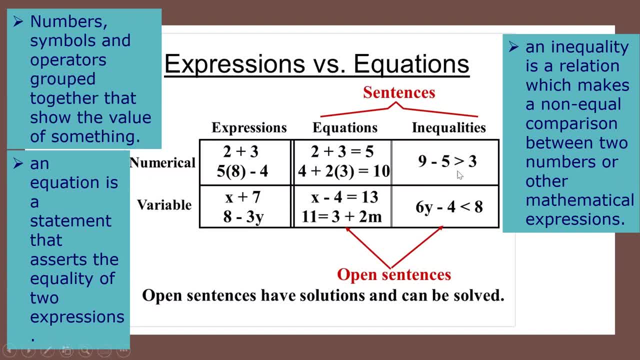 It uses inequality symbols such as greater than, less than, the less than or equal to and the greater than or equal to. So here, in this example, the expression 9 minus 5 is being compared to 3.. As 9 minus 5 is greater than 3.. 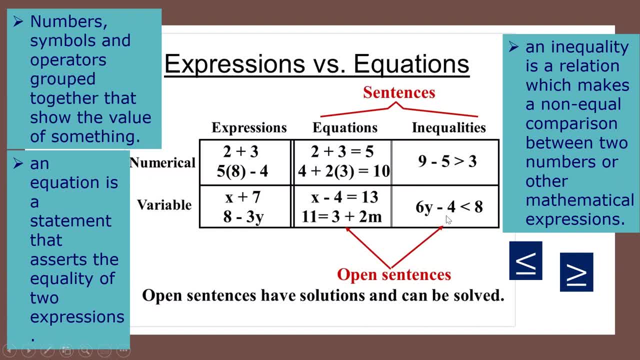 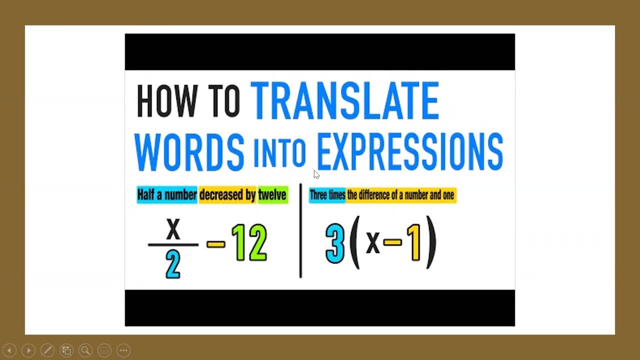 Same as this. The expression 6y minus 4 is being compared to 8.. As 6y minus 4 is less than 8.. Now how are we going to translate words into expressions, equations and inequalities? Now we need these synonyms. 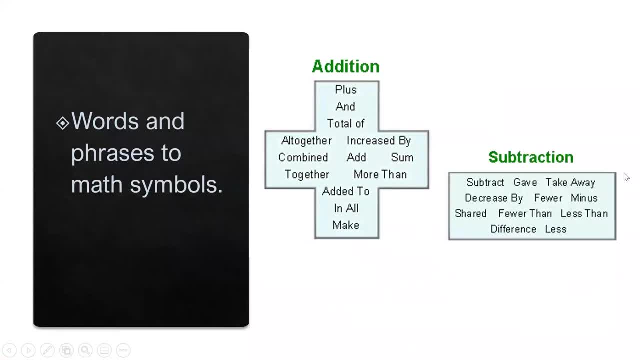 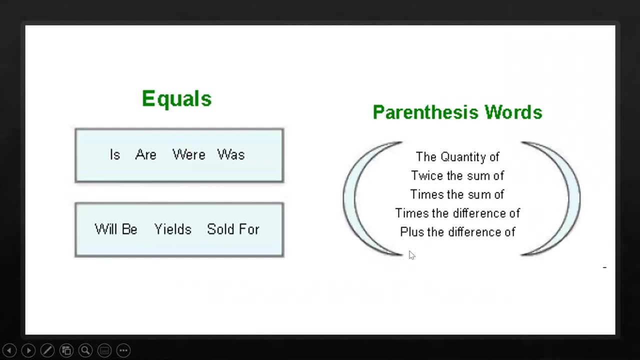 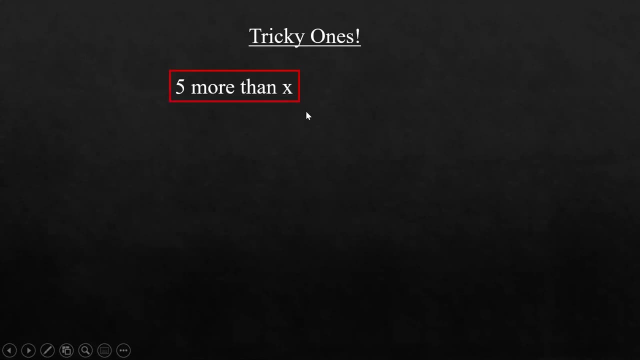 For addition, take note of these words: For subtraction, For multiplication, For division, For equals, For parentheses. Now remember these tricky ones: 5 more than x. The word done means we're going to switch position: The 5 and the x. 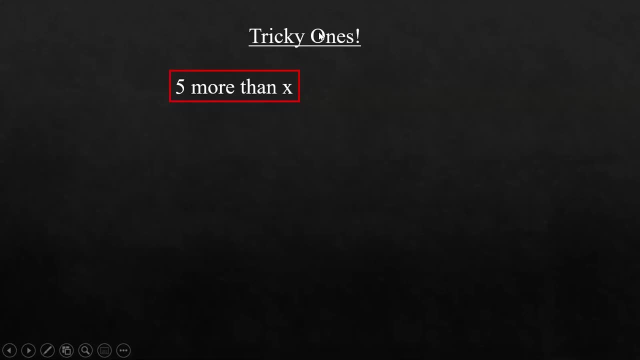 Because if we're going to translate this literally, this will become: 5 more than means plus and x, But the word done it means we're going to switch position, Because 5 more than x it means that 5 is being added to x. 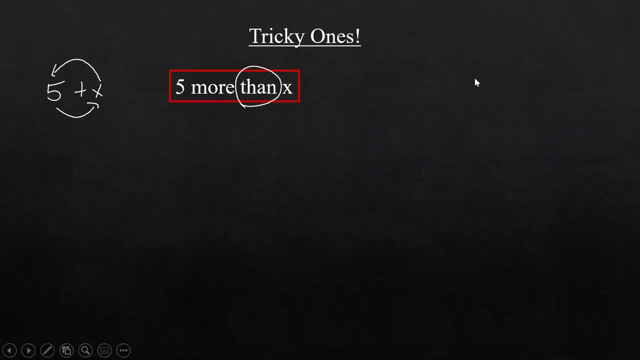 So this is x plus 5.. Not this. Okay, Now, 5 is more than x. So take note of the phrase. Take note of the phrase: Is more than, Is more than means comparison. 5 is being compared to x. 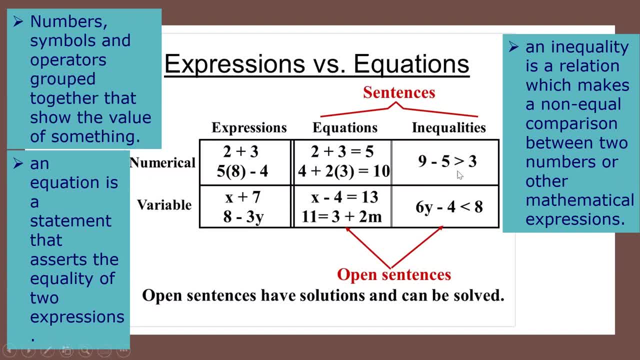 It uses inequality symbols such as greater than, less than, the less than or equal to and the greater than or equal to. So here, in this example, the expression 9 minus 5 is being compared to 3.. As 9 minus 5 is greater than 3.. 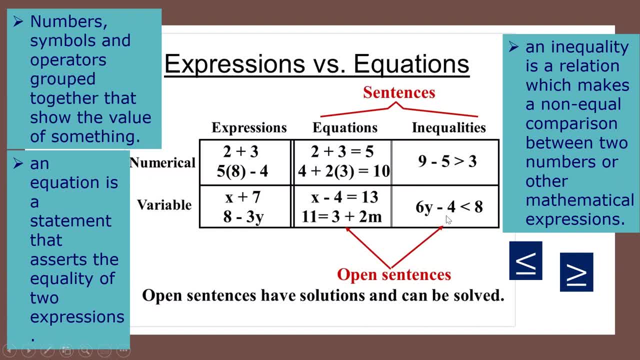 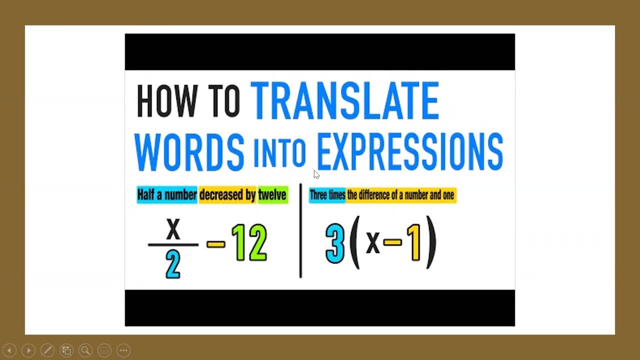 Same as this. The expression 6y minus 4 is being compared to 8.. As 6y minus 4 is less than 8.. Now how are we going to translate words into expressions, equations and inequalities? Now we need these synonyms. 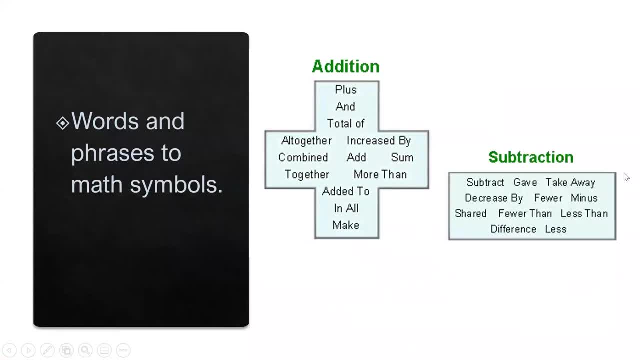 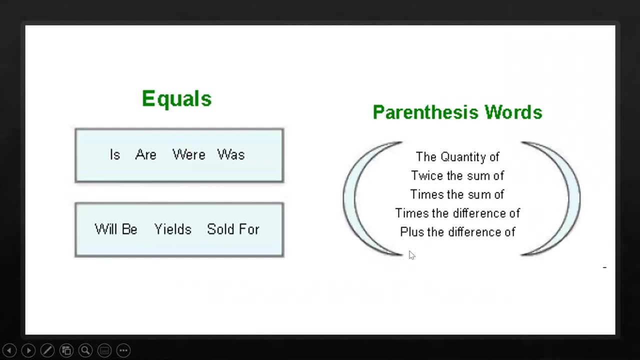 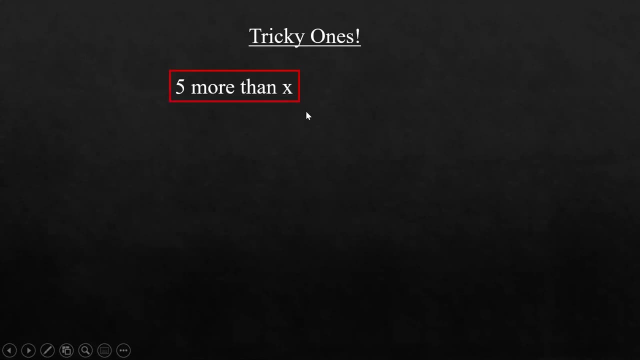 For addition, take note of these words: For subtraction, For multiplication, For division, For equals, For parentheses. Now remember these tricky ones: 5 more than x. The word done means we're going to switch position: The 5 and the x. 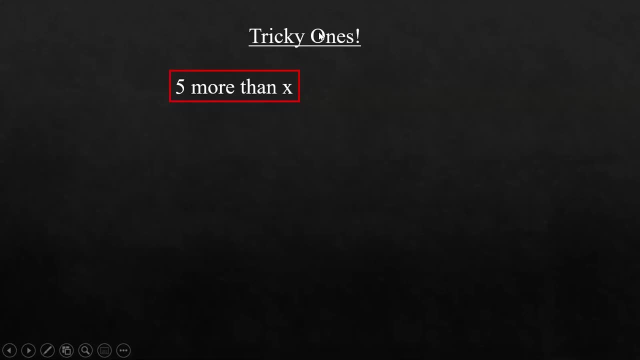 Because if we're going to translate this literally, this will become: 5 more than means plus and x, But the word done it means we're going to switch position, Because 5 more than x it means that 5 is being added to x. 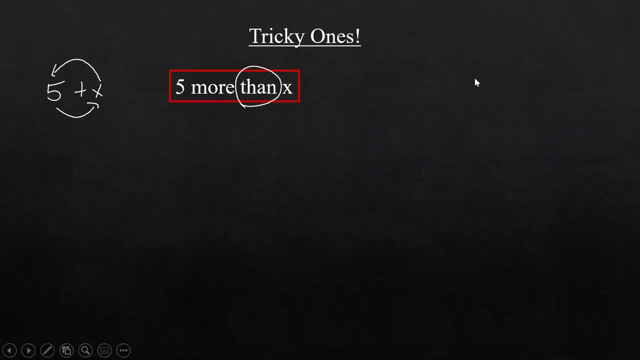 So this is x plus 5.. Not this. Okay, Now, 5 is more than x. So take note of the phrase. Take note of the phrase: Is more than, Is more than means comparison. 5 is being compared to x. 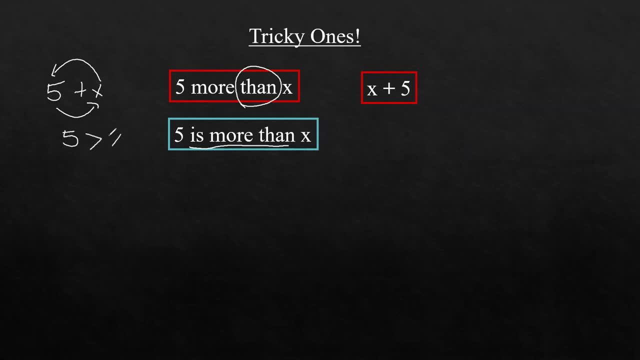 As 5 is more than x, So that is 5 is greater than x. Now here 5 less than x, So meaning 5 is being subtracted from x, So that is x minus 5.. Not 5 minus x. 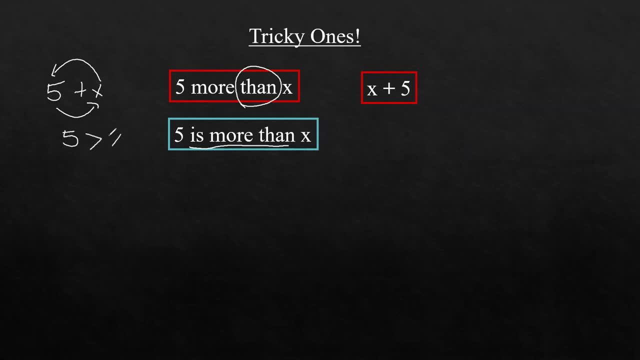 As 5 is more than x, So that is 5 is greater than x. Now here 5 less than x, So meaning 5 is being subtracted from x, So that is x minus 5.. Not 5 minus x. 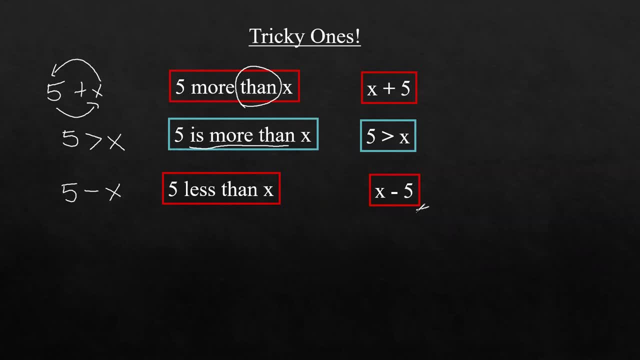 Not this. This is the correct one. We need to switch position, Especially for subtraction, Because subtraction is not commutative. Now okay. Next, We have 5 subtracted from x, So x minus 5.. And this 5 is less than x. 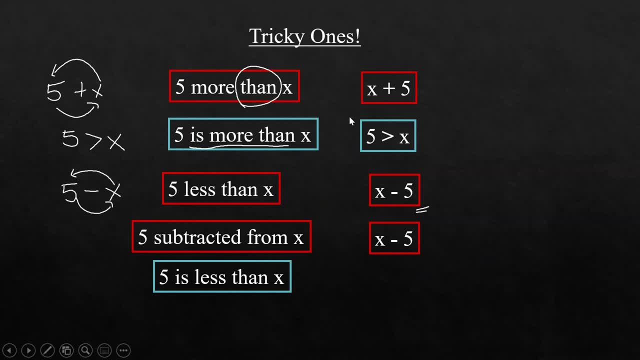 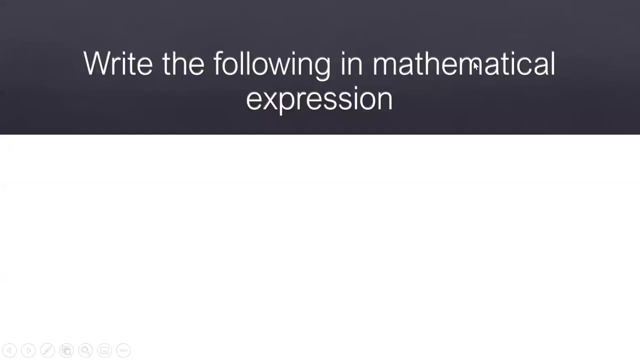 5 is being compared to x, So that is 5 is being compared to x as less than, So that is x, 5 less than x. Okay, Let's proceed. So let's have the following examples: 45 minus y. 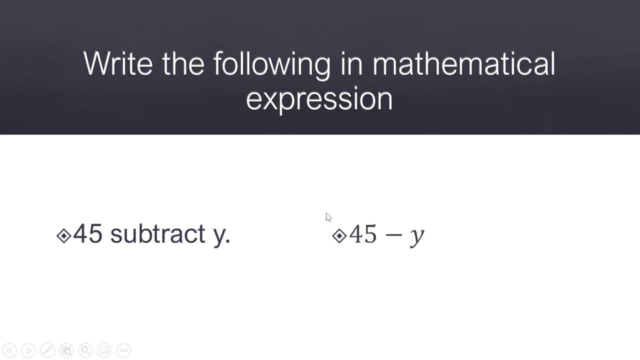 So simply 45 minus y, 45 subtract y, So simply 45 minus y. The product of 5 and p Product means multiply, So this is 5p, 50 decreased by a number. x. Decreased means minus. 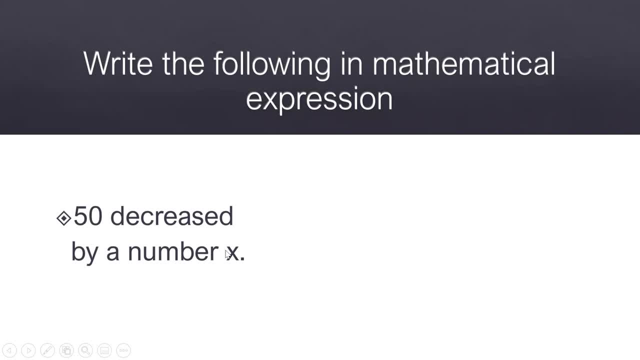 There is no word done, So we are not going to switch the position of 15x. So this is just 50 minus x. Next, 3 added to the product of 5 and n. Product means times 3 is added to the product of 5 and n. 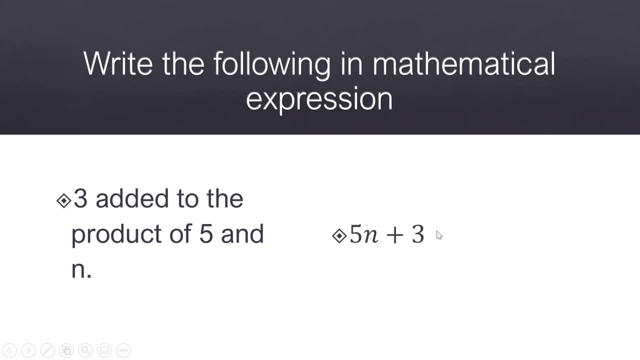 So this is 5n plus 3.. Next, The quotient of 7 and a number x less 2.. So quotient means divide 7.. Quotient means divide. 7 is 7.. A quotient of 7 and a number x less 2.. 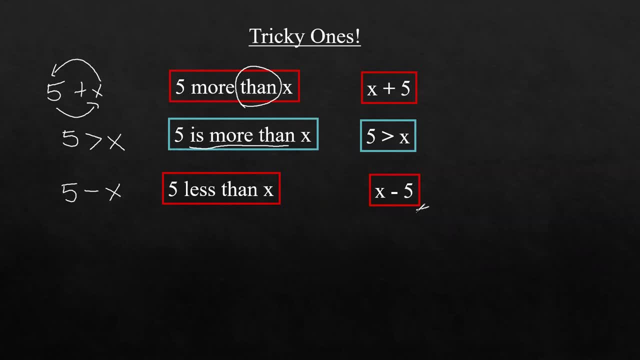 Not this. This is the correct one. We need to switch position, Especially for subtraction, Because subtraction is not commutative. Now okay. Next, We have 5 subtracted from x, So x minus 5.. And this 5 is less than x. 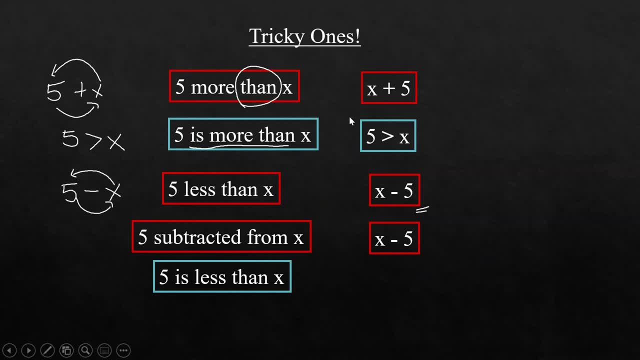 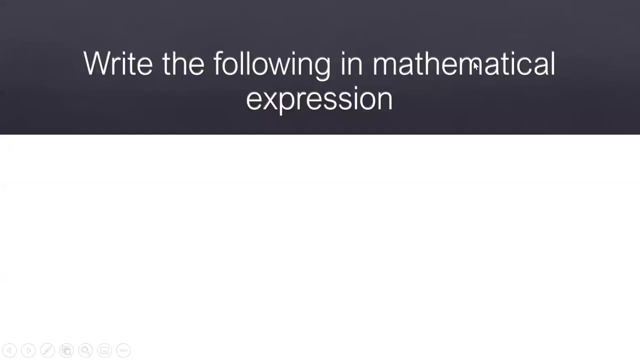 5 is being compared to x, So that is 5 is being compared to x as less than, So that is x, 5 less than x. Okay, Let's proceed. So let's have the following examples: 45 minus y. 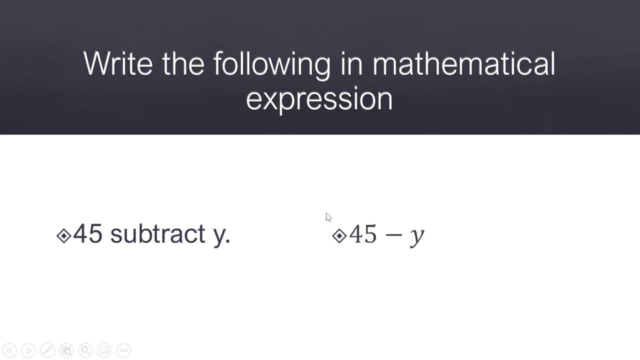 So simply 45 minus y, 45 subtract y, So simply 45 minus y. The product of 5 and p Product means multiply, So this is 5p, 50 decreased by a number. x. Decreased means minus. 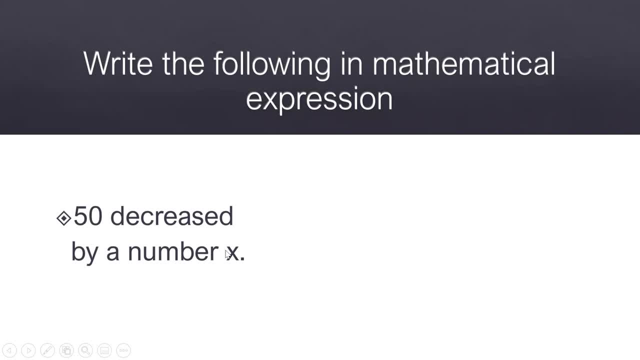 There is no word done, So we are not going to switch the position of 15x. So this is just 50 minus x. Next, 3 added to the product of 5 and n. Product means times 3 is added to the product of 5 and n. 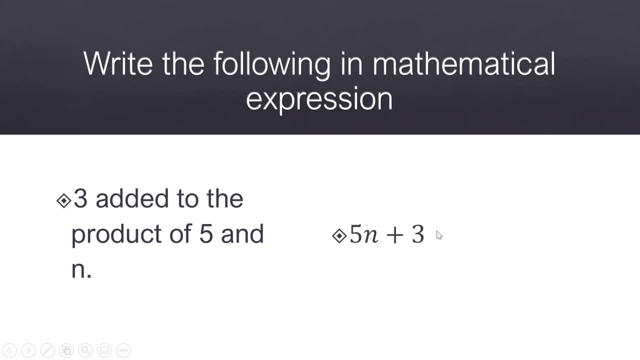 So this is 5n plus 3.. Next, The quotient of 7 and a number x less 2.. So quotient means divide 7.. Quotient means divide. 7 is 7.. A quotient of 7 and a number x less 2.. 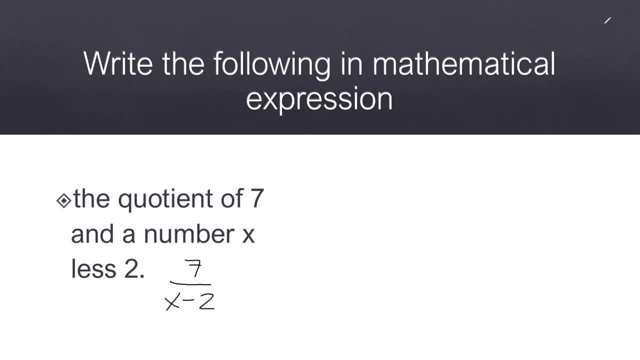 So x minus 2.. Okay, Next, 4 less than 3 times t, So 3 times t minus 4.. So this is 4.. Less than means minus, But there is the word done Meaning. we are going to switch position. 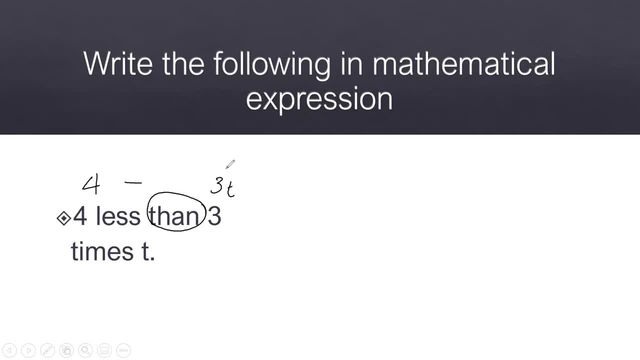 3 times t means 3t, Switch position because of the word done. So this is equal to 3t minus 4.. Okay, Meaning 4 is being subtracted from 3 times t, Next 5 times the sum of y and 4.. 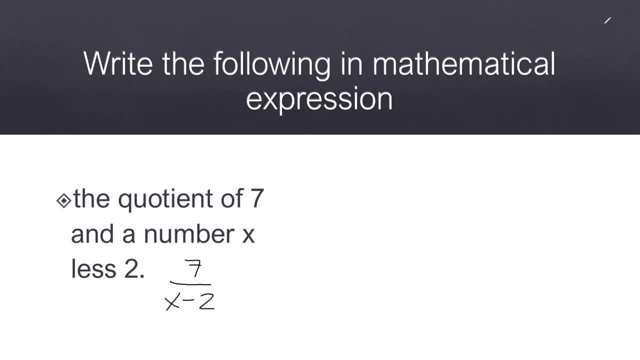 So x minus 2.. Okay, Next, 4 less than 3 times t, So 3 times t minus 4.. So this is 4.. Less than means minus, But there is the word done Meaning. we are going to switch position. 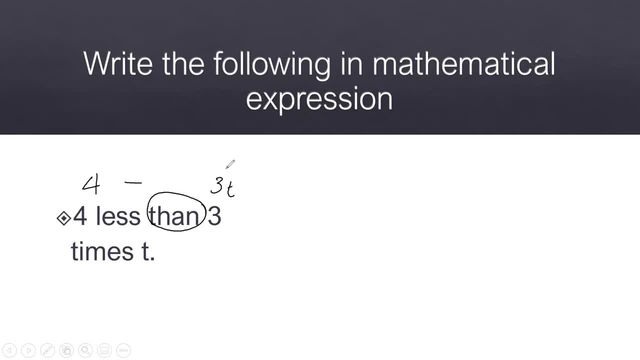 3 times t means 3t, Switch position because of the word done. So this is equal to 3t minus 4.. Okay, Meaning 4 is being subtracted from 3 times t, Next 5 times the sum of y and 4.. 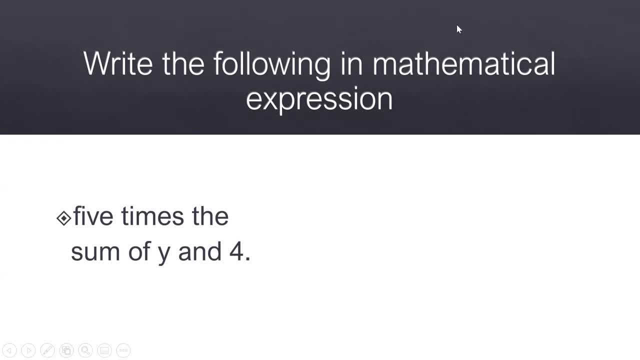 The sum of, Okay, The sum of. There is parenthesis, Right, Remember the synonyms: 5 times the sum of y and 4.. Okay, So 5 times the sum of y and 4.. Next, we have 5 less than twice the sum of. 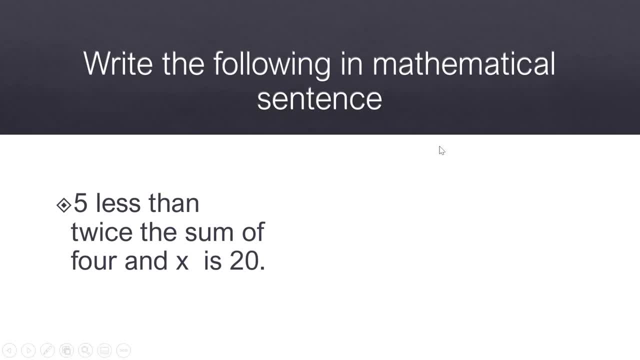 The sum of again. Meaning there is parenthesis, Okay, Again. Is less than Ah. 5 less than There is no is between 5 and less. So meaning this is subtraction, So done. meaning we are going to switch positions. 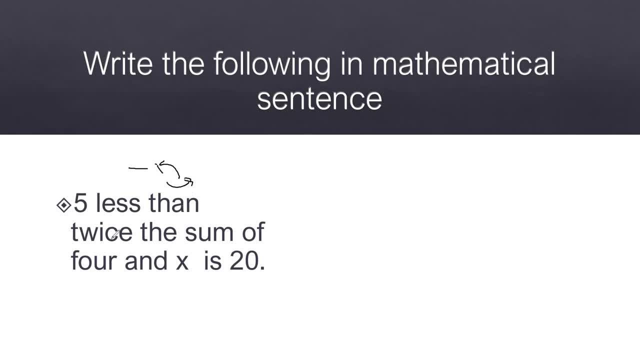 Okay, Switch Twice times 2.. The sum of meaning parenthesis, and there is plus, Is means 20.. So this is what: 2 times 4 plus x minus 5 is equal to 20.. So 5 less than twice the sum of 4 and x is 20.. 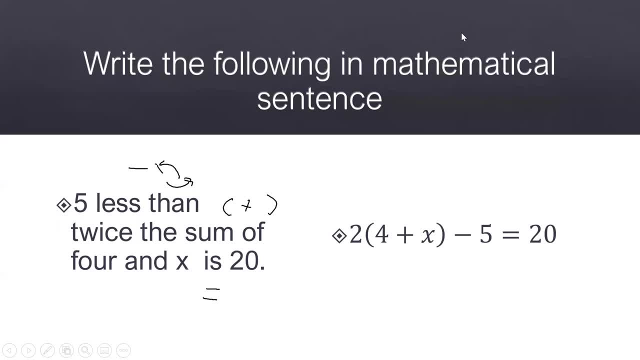 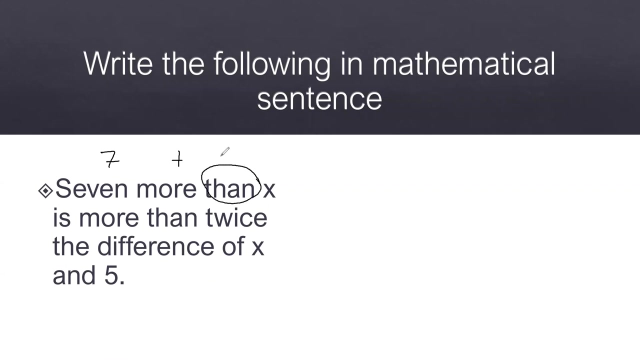 Okay, Next, 7 more than x is more than twice the difference of 5 and of x and 5.. So 7 more than means plus, But done means we are going to switch positions. Is more than Meaning comparison. Meaning comparison. 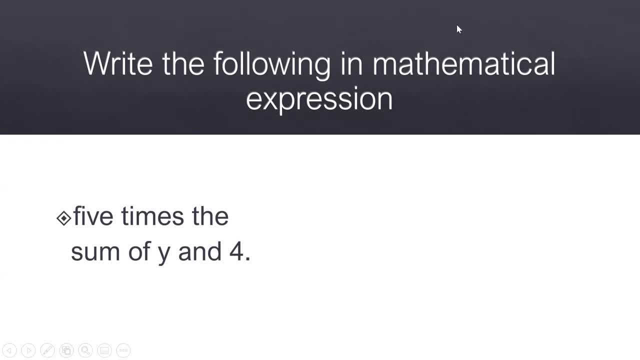 The sum of, Okay, The sum of. There is parenthesis, Right, Remember the synonyms: 5 times the sum of y and 4.. Okay, So 5 times the sum of y and 4.. Next, we have 5 less than twice the sum of. 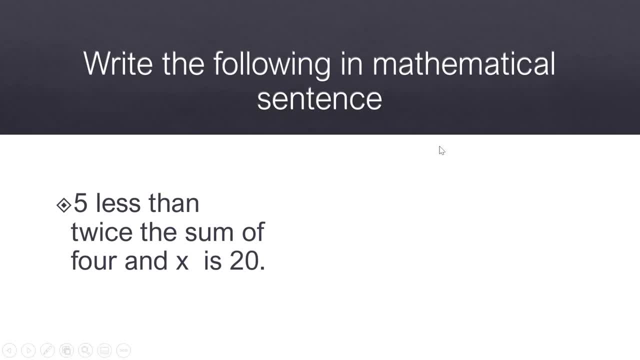 The sum of again. Meaning there is parenthesis, Okay, Again. Is less than Ah. 5 less than There is no is between 5 and less. So meaning this is subtraction, So done. meaning we are going to switch positions. 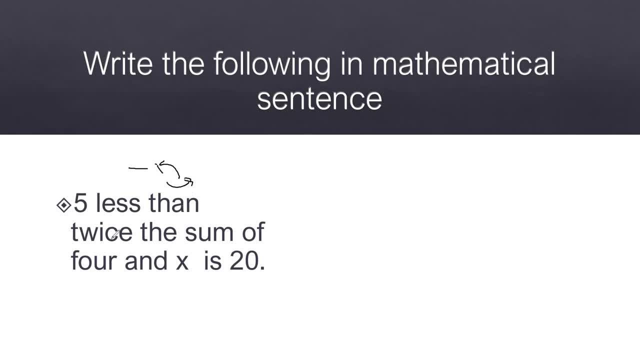 Okay, Switch Twice times 2.. The sum of meaning parenthesis, and there is plus, Is means 20.. So this is what: 2 times 4 plus x minus 5 is equal to 20.. So 5 less than twice the sum of 4 and x is 20.. 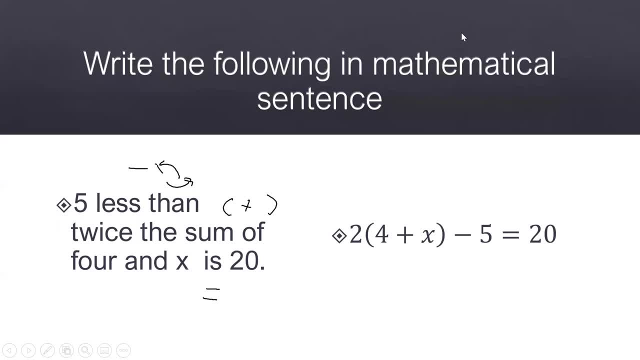 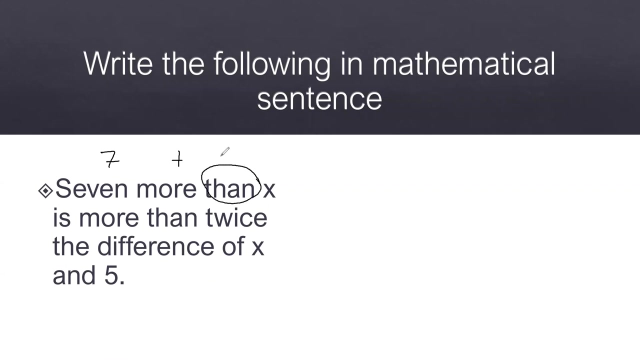 Okay, Next, 7 more than x is more than twice the difference of 5 and of x and 5.. So 7 more than means plus, But done means we are going to switch positions. Is more than Meaning comparison. Meaning comparison. 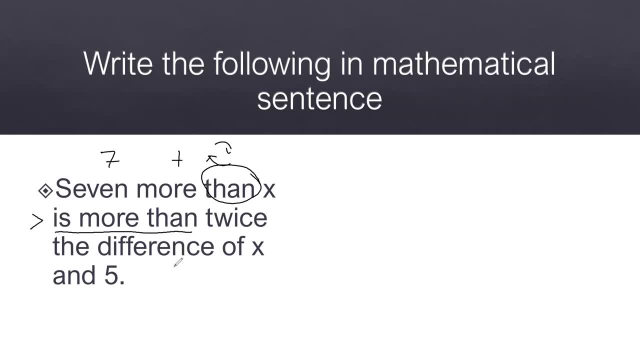 This is greater than Twice the difference of minus x and 5.. Difference of meaning: there is parenthesis here. Remember the synonyms. So this is x plus 7.. Okay Is greater than the difference Twice the difference of x and 5.. 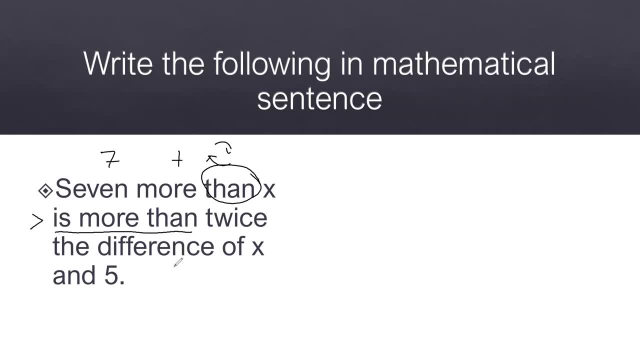 This is greater than Twice the difference of minus x and 5.. Difference of meaning: there is parenthesis here. Remember the synonyms. So this is x plus 7.. Okay Is greater than the difference Twice the difference of x and 5.. 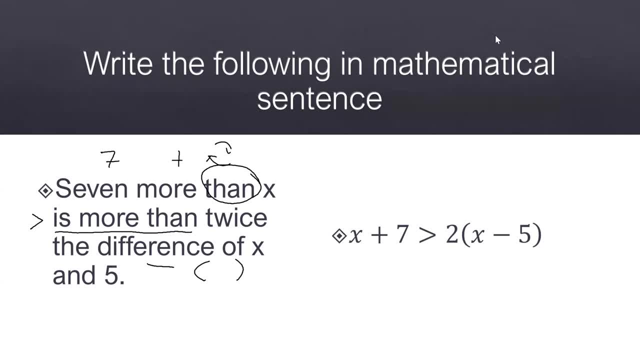 Next, The quotient of x and 4 is less than the product of 5 and x. The quotient means divide. The quotient of x and 4 is means equal 6 less than. So less than means minus Done means we are going to switch positions. 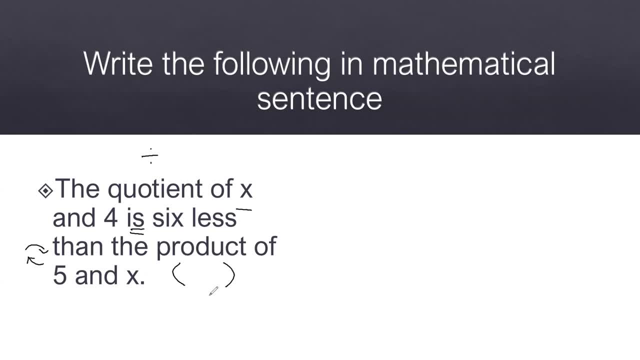 Product of, Product of means parenthesis. Or if you are going to write parenthesis, Just write this: 5x, Okay. So that is The quotient of x, and 4 is 5 less than. Okay Is 6 less than. 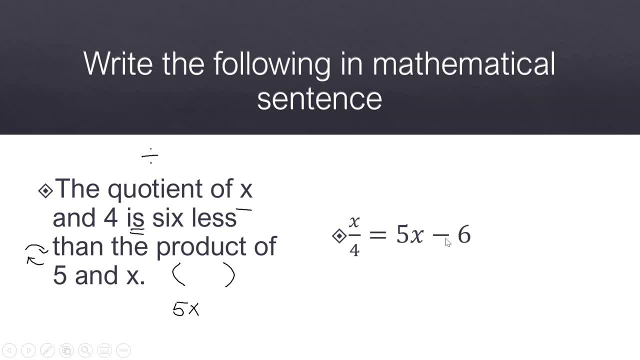 Okay, Is 6 less than 5 and x. The product of 5 and x. Next, 8 less than x is less than 4 less x. Okay, The quotient of x and 4 is 8 less than, meaning minus. 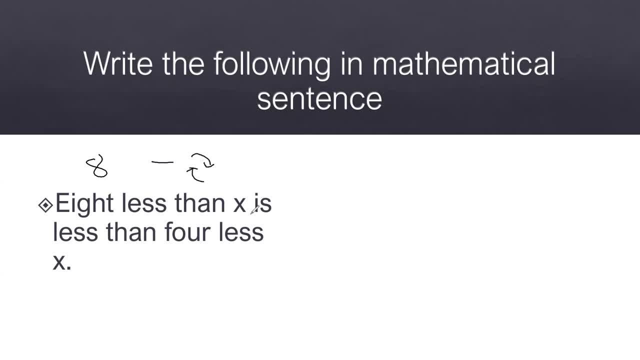 Done means switch. position Is less than means comparison. Less than 4 less x. So 4 less means minus x. So this is what x minus 8 is less than 4 minus x. Okay, Okay, So 8 less than x. 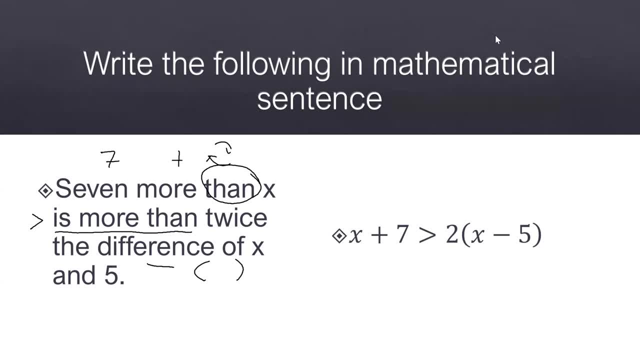 Next, The quotient of x and 4 is less than the product of 5 and x. The quotient means divide. The quotient of x and 4 is means equal 6 less than. So less than means minus Done means we are going to switch positions. 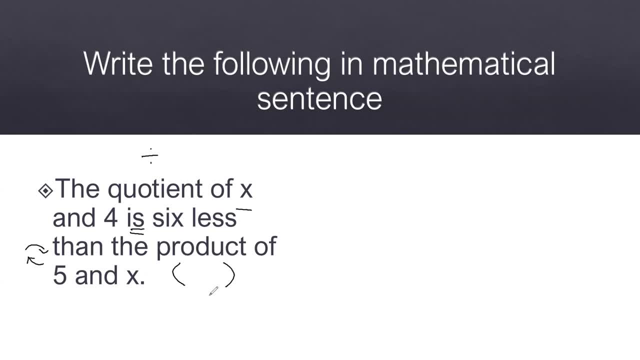 Product of, Product of means parenthesis. Or if you are going to write parenthesis, Just write this: 5x, Okay. So that is The quotient of x, and 4 is 5 less than. Okay Is 6 less than. 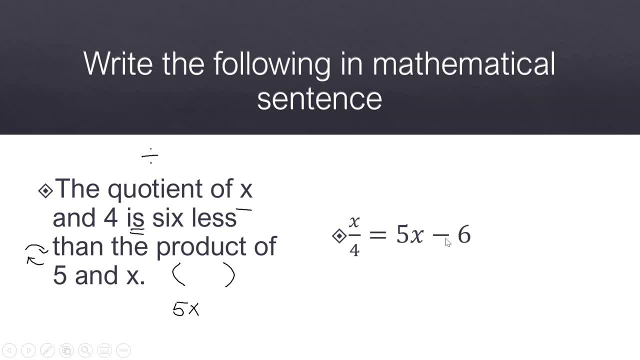 Okay, Is 6 less than 5 and x. The product of 5 and x. Next, 8 less than x is less than 4 less x. Okay, The quotient of x and 4 is 8 less than, meaning minus. 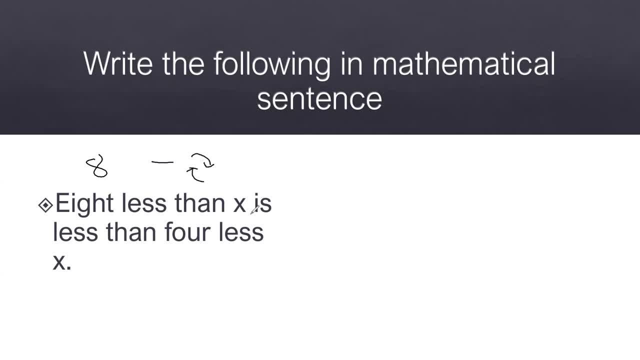 Done means switch. position Is less than means comparison. Less than 4 less x. So 4 less means minus x. So this is what x minus 8 is less than 4 minus x. Okay, Okay, So 8 less than x. 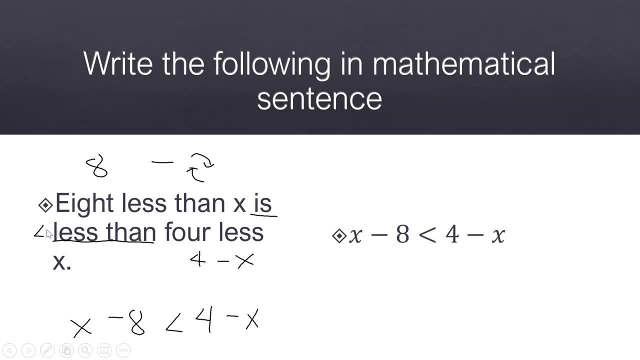 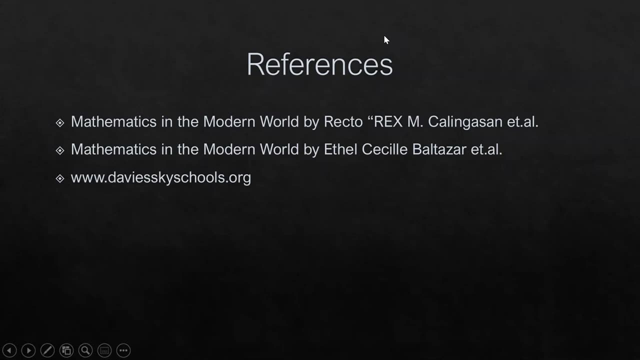 So switch position Is less than meaning comparison: Less than 4 less x. Okay, So thank you. Here are my references.